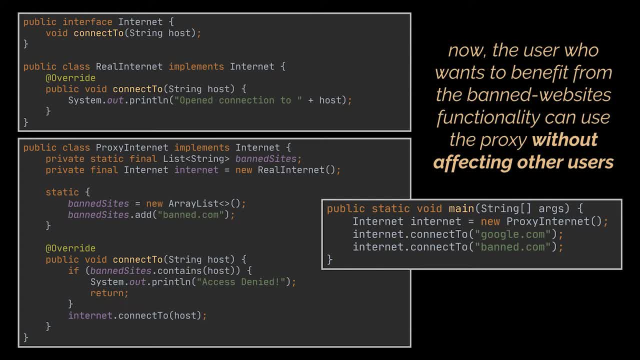 of an intermediary server, a proxy that checks the user requests among a list of banned websites and if the user tries to access any of them, they will be able to access them all over the internet. If we restrict access to these websites, an access denied error will pop up, for example. 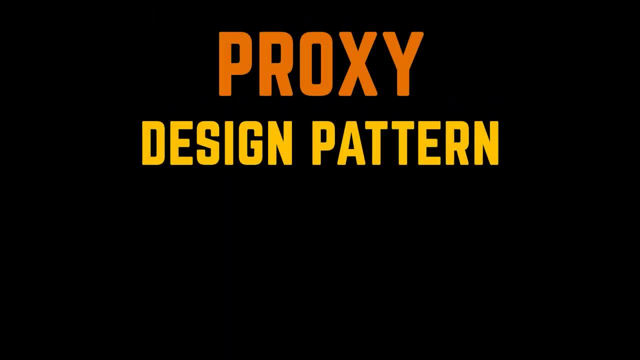 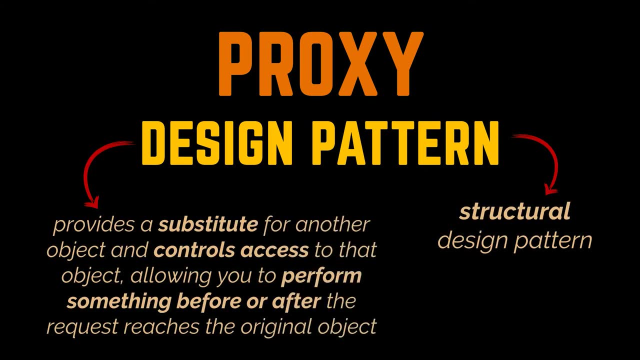 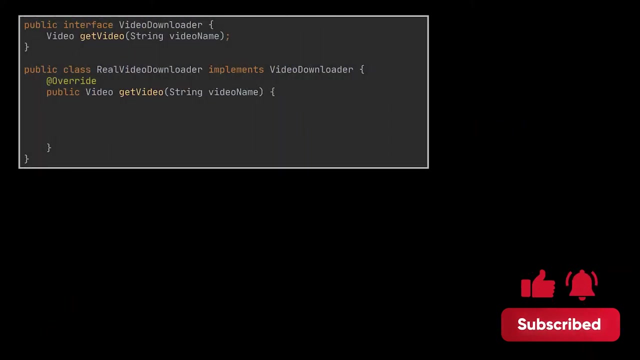 See, that is exactly what the proxy pattern is all about. This pattern is a structural design pattern that lets you provide a substitute or placeholder for another object. It controls access to the original object, allowing you to perform something before or after the request reaches the original object. Let's take another example: Speed of access and caching, Suppose. 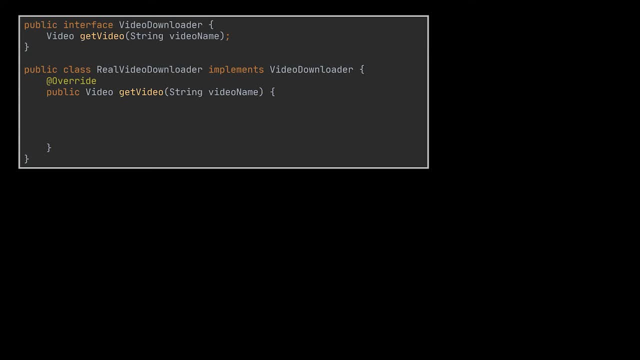 you're a downloader class. This class takes the name of the video you want to download, then connects to YouTube, downloads the video, retrieves all its metadata and the download location corresponding to that video, and returns with all this info to you using the. 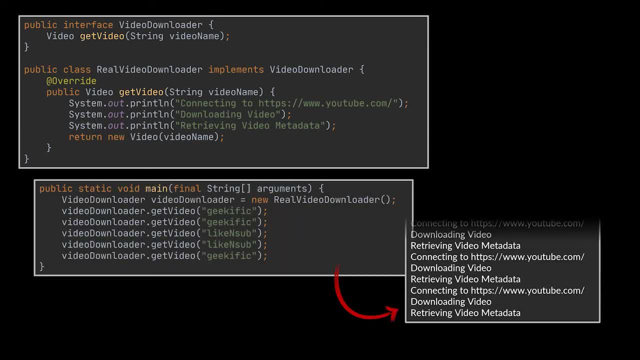 video object. you see Now notice how, every time we need a particular video, that video gets downloaded all over again, even if it was previously downloaded. To avoid this, what we need is some caching mechanism that will allow us to access the video we want. 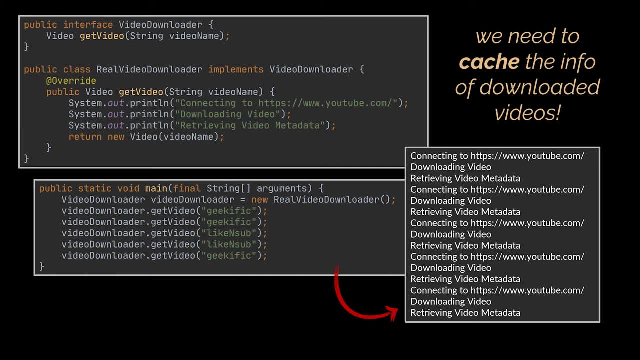 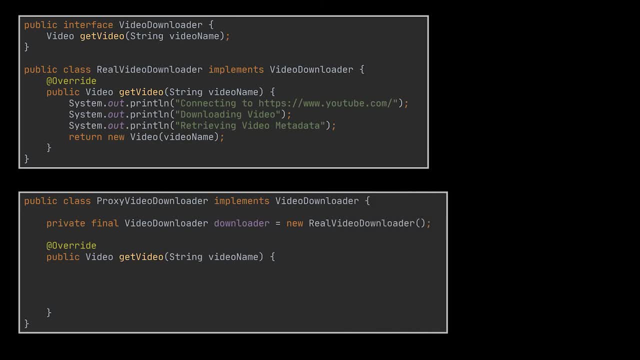 to download and store the information related to videos we already downloaded, sparing us the need to do it again. The proxy class you see here will provide exactly this functionality. The proxy will implement the same interface as the original downloader and will delegate to the original service all the work. However, it will keep track of the downloaded files. 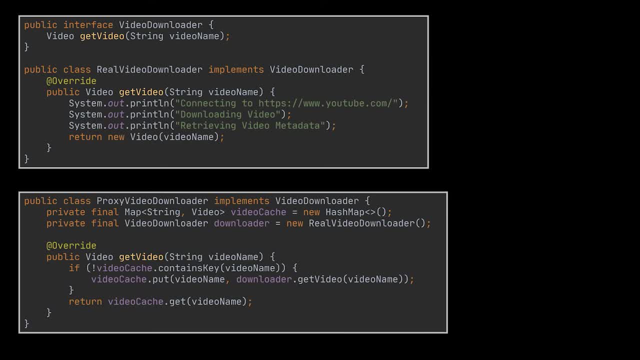 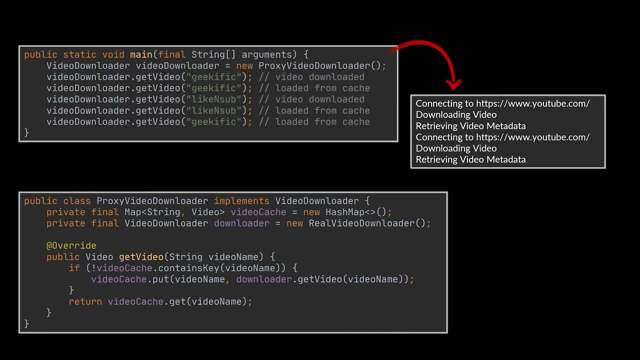 using a hash map and will return the cached result to the user if they request the same video multiple times. Going back to the same client call we had, you can clearly see that the two videos requested are now being downloaded once each, instead of five times as we previously saw. 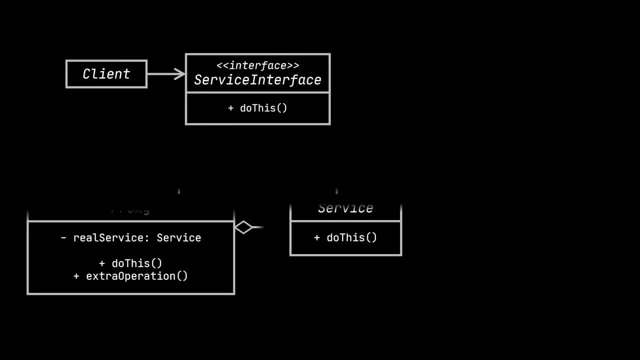 Okay, let's go ahead now and take a look at the structure or class diagram of the proxy pattern, while trying to relate it to the internet and caching examples. we just implemented First the service interface, which was represented by both the internet and video downloader.